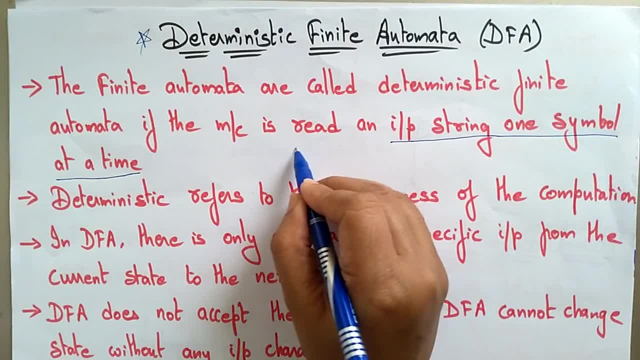 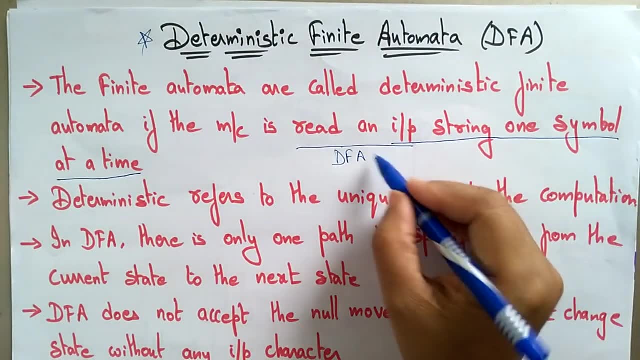 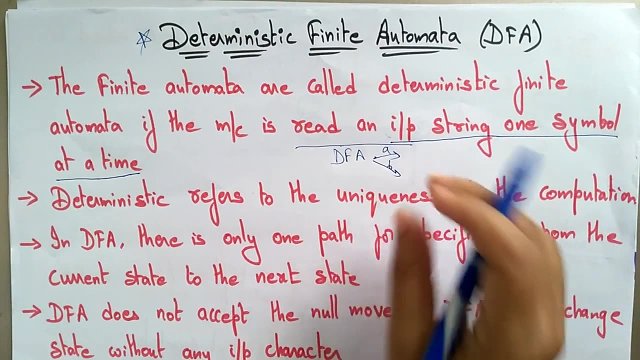 non-deterministic. Okay so here DFA is going to read the input symbol, that is, the input string. one symbol at a time. Suppose, if it is reading A means it will read only one input string at a time And B means it can read only B input string. one symbol, that is, a. one symbol at a time it can read. Okay so. 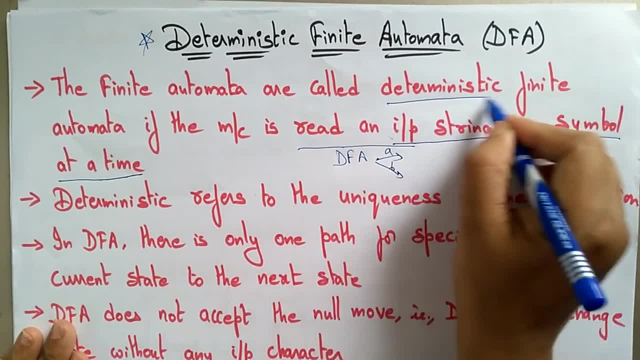 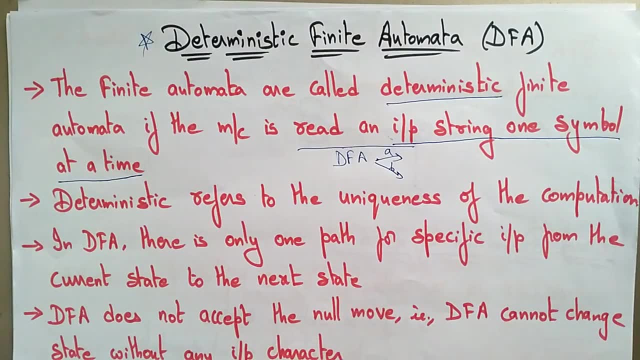 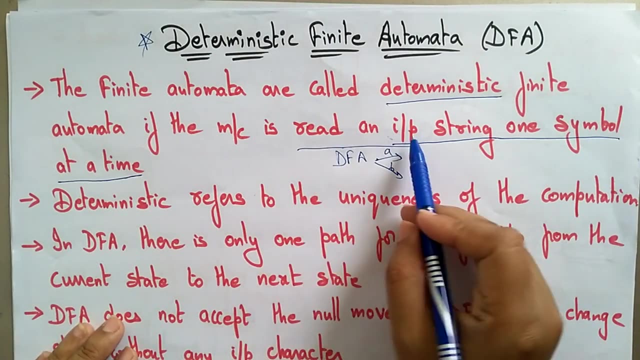 there is no multiple paths, only the fixed path. Deterministic means fixed. Only one way is there? Okay, It's a one-way solution. Either it has to be accepted or it has to be the rejected. Okay, so the deterministic finite automata is he. it is an automata if the machine is read an input string. 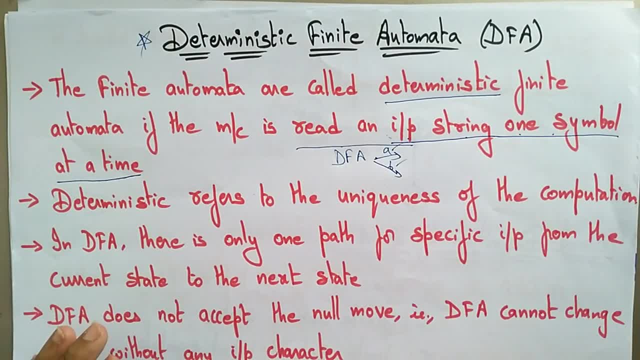 one symbol, the one symbol at a time, So that the word deterministic it's a fixed one. either it can be. it has only one thing, that is, it has to be accepted or it has to be rejected. There is no alternate solution in the deterministic finite automata. 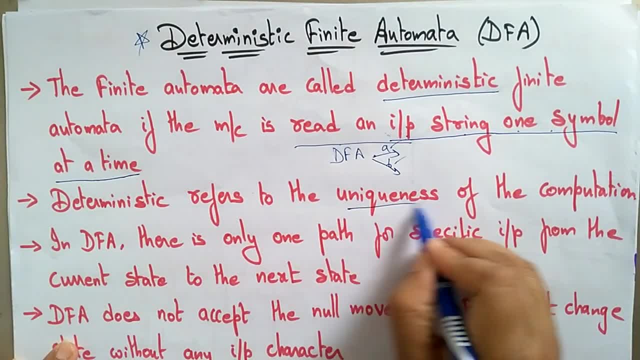 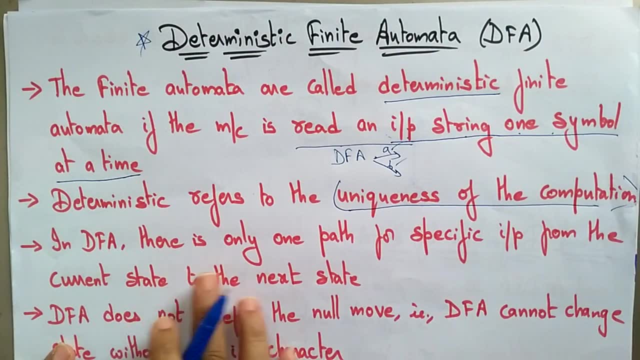 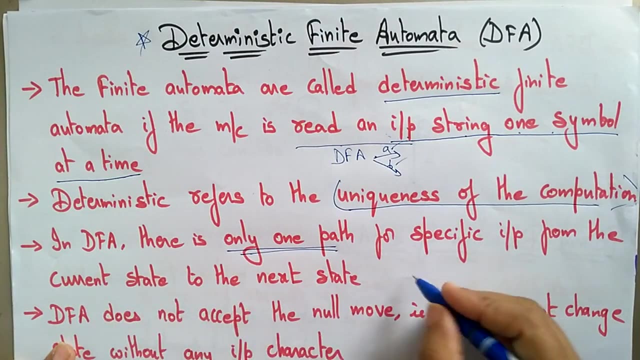 Deterministic refers to the uniqueness of the computation. So that's what I said. now It is- and uniqueness of the computation. In DFA there is only one path. there is only one path for specific input from the current state to the next state. Suppose, if I wants to go from A to B, okay there. 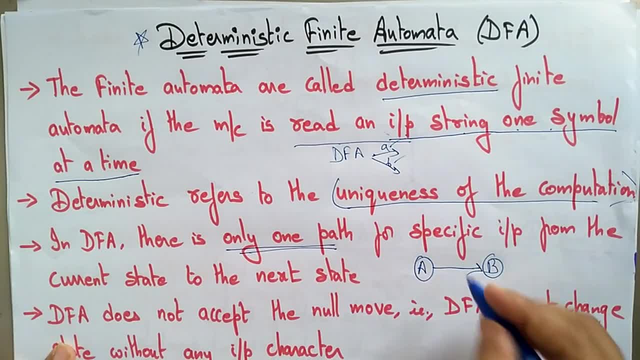 is only one path will be there. If the input zero is there, it has to go. only the zero can be go to, only to the B right. That is the�. This is everybody I know. okay, The input one is this: only the mom. particular path will go to B If population Вот. you know that. Okay, So that is the prom domain. So this would be clarifying which is the leading element determining what detriministic refers to: the uniqueness of the computation. So that is that what I've said. now, It is an uniqueness of the computation. 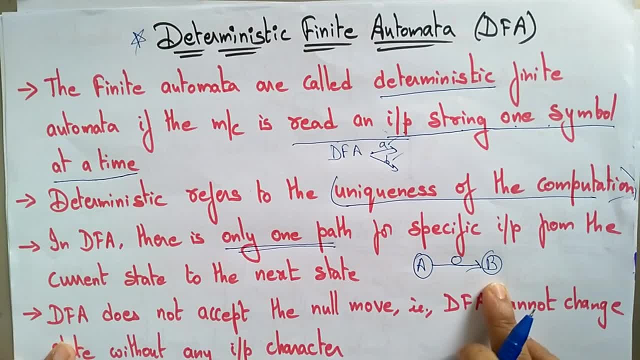 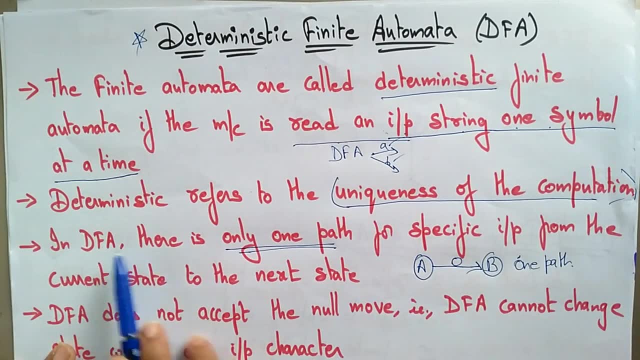 only to the B, only to the current state, to the next state. That is only one path, is there? Only one path? So remember that In DFA there is only one path for specific input. So this is a specific input, A specific input from the current state to the next state. 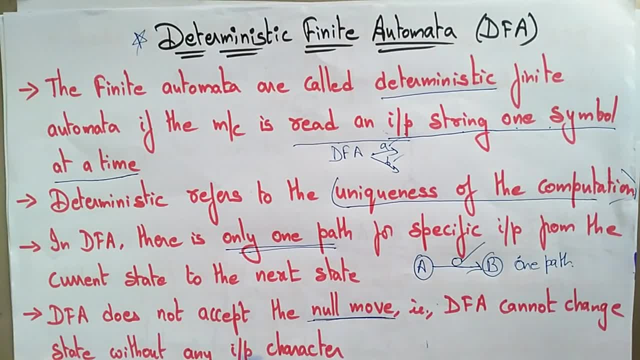 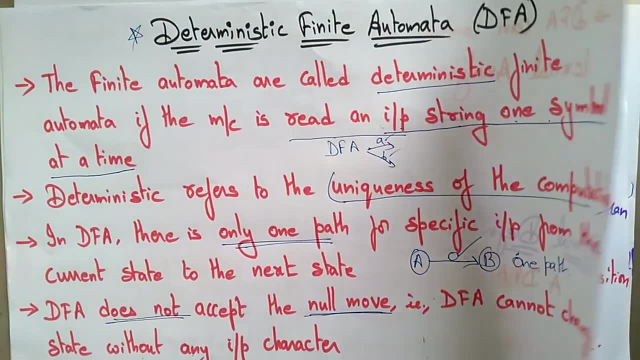 DFA does not accept the null moves, So it does not accept the. it does not accept the null moves, That is, DFA cannot change state without input character. So if input character is there, then only it can change to the another state. If suppose input character is not. 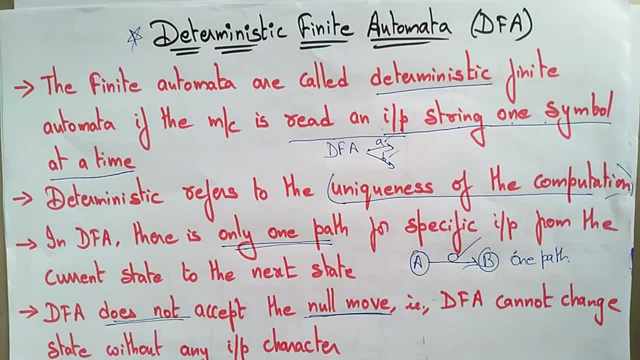 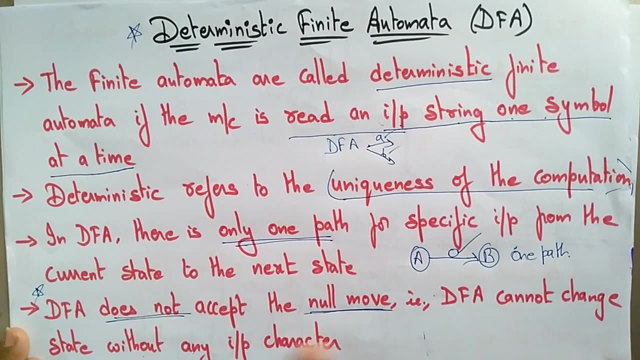 input character is not present, it does not moves to the next state Only. it will be stay in that state only and string will be rejected. Okay, The automata will be rejected. Remember this: A DFA does not accept the null moves, That is, DFA cannot change state without any. 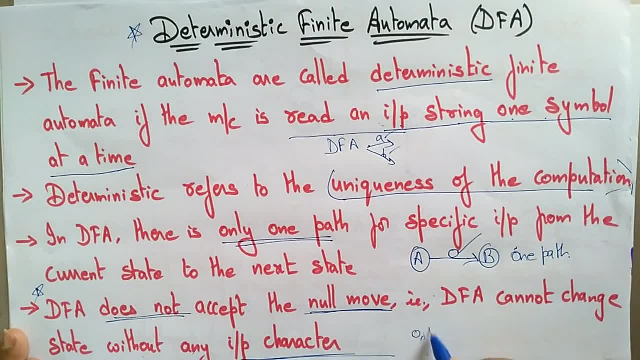 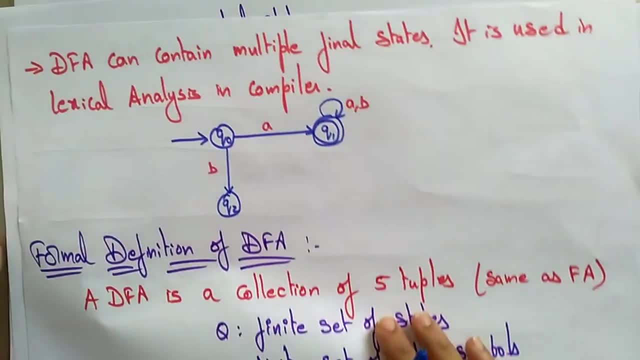 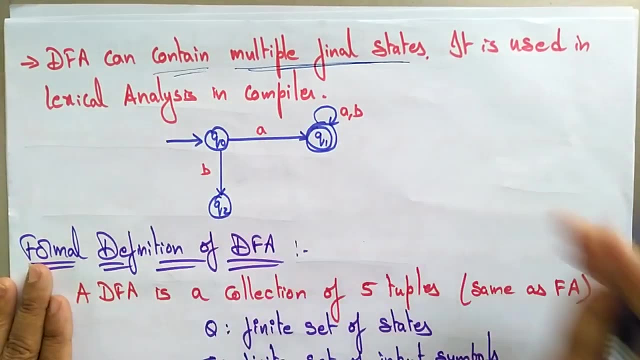 input, Whenever the input character- either 0 or 1 or A or B, anything, Okay, If any input character is present, then only it moves to the next state. DFA can contain multiple final states. So this is one thing Here you have to remember: that DFA can have multiple final states. That is. 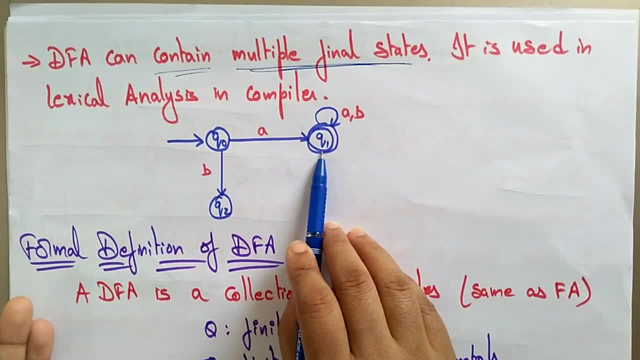 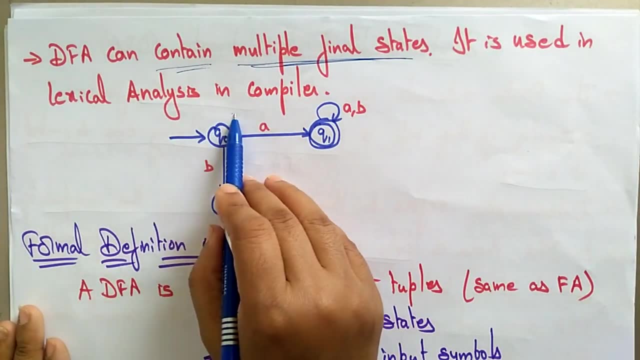 either one or more. Here. in this example I have taken only one final state. So in DFA there are multiple final states And it is used in in the compiler. So where the DFA will be used? The DFA will be used in the lexical analysis in. 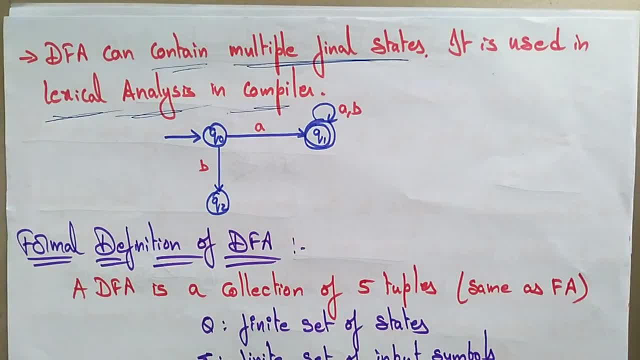 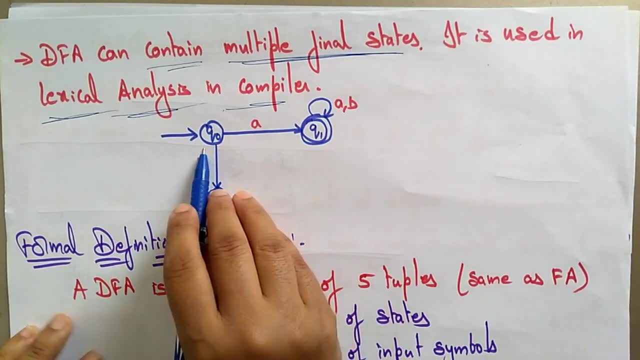 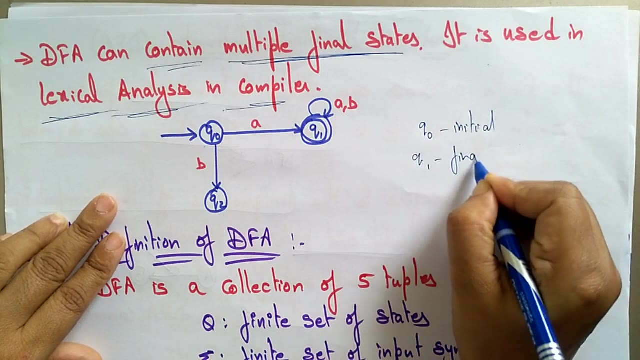 the compiler, In the compiler. the first phase is the lexical analysis phase, So in that phase the finite automata, deterministic finite automata, will be used. So here you can see: Q0 is the initial state, Initial state, And Q1 is the final state And the remaining or the intermediate state. 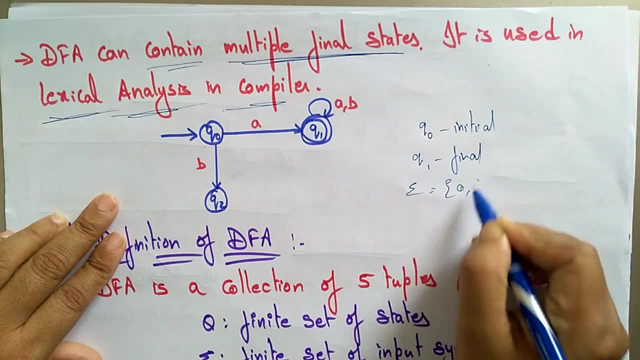 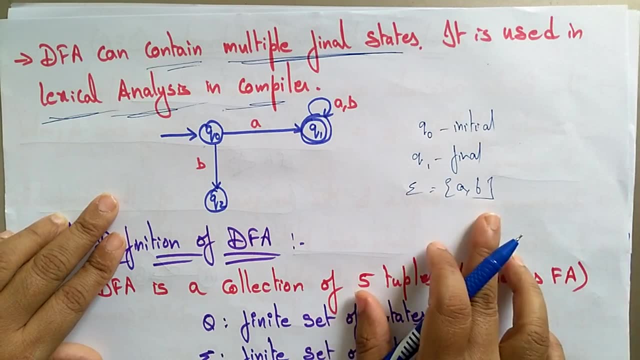 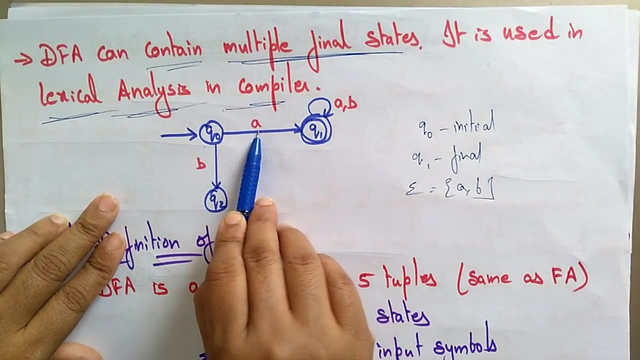 And the input strings, that is inputs, are A, B. So here this DFA is constructed with a set of strings, A, symbols, A, B. Okay, So you can observe, here Each state is moving to another state with the help of input only. There is no without, it is without epsilon modes. So here on Q0, on A goes. 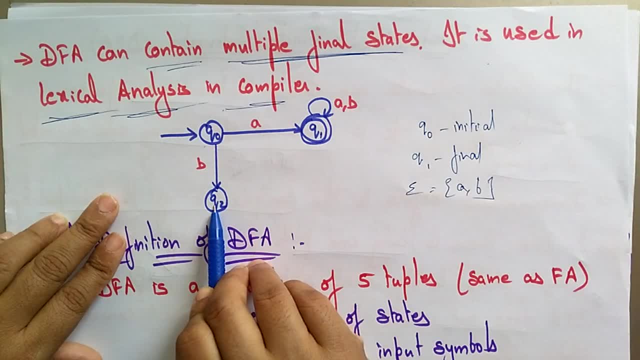 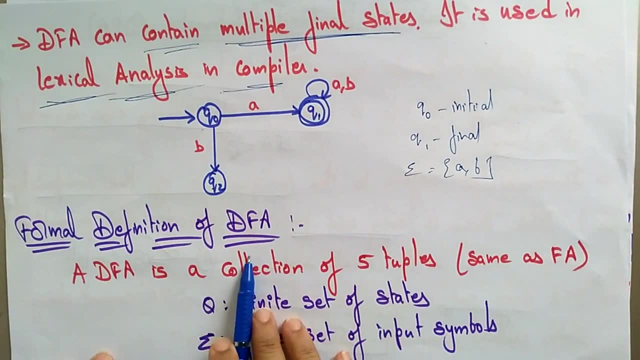 to Q1.. And Q0 on B goes to Q2 only. Okay, So only one input at a time. So this is DFA. Now let's see the formal definition of DFA. A DFA is a collection of 5-tuple, So it's- the definition is same as the finite automata Here, the 5-tuple Q. 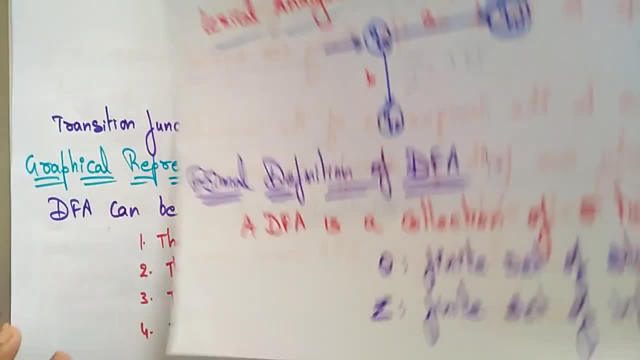 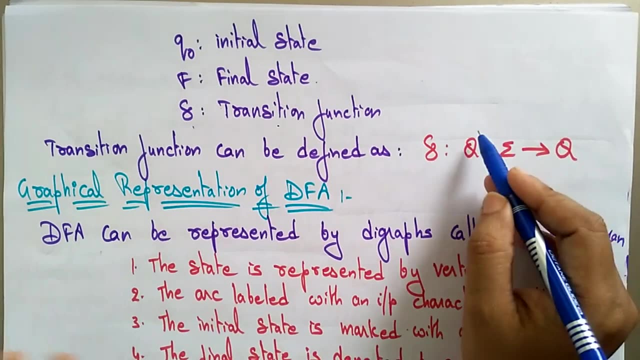 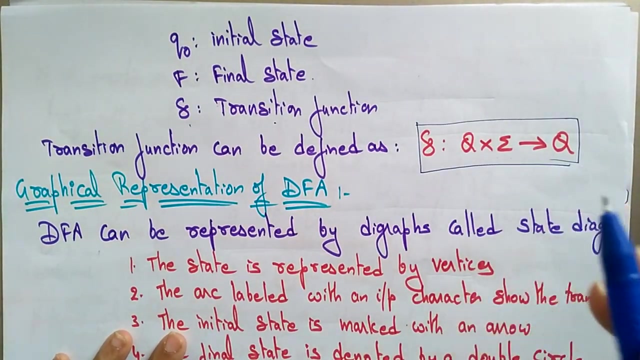 that is, Q is the finite set of states And sigma is the finite set of input symbols And Q0 is the initial state, F is the final state And delta is the transition function. So where the transition function is defined as delta is Q into sigma, is tends to, Q Means the 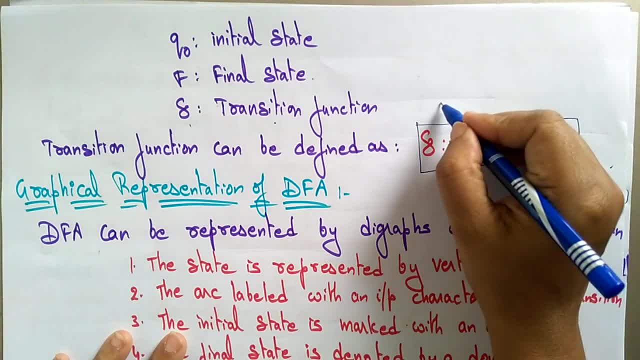 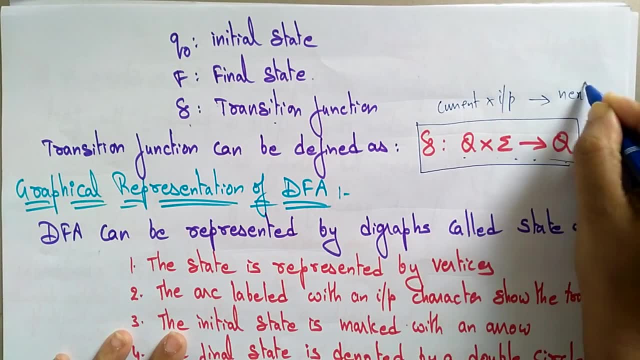 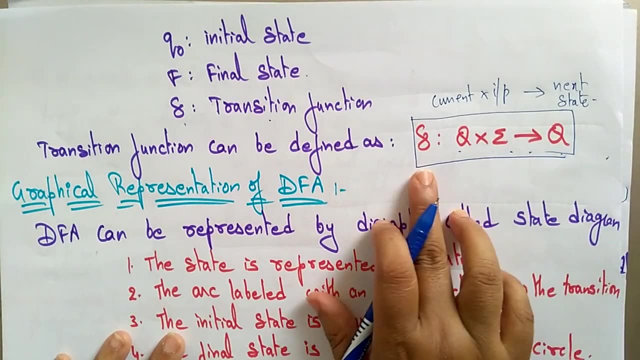 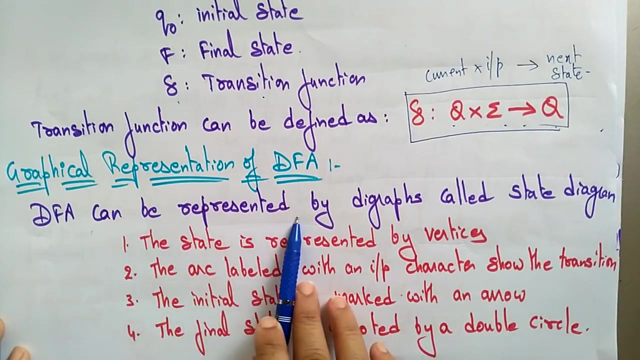 state with input symbol leads to the next state. current state input symbol gives the next state: okay. current state in input symbol leads to the next state. that is the definition of the transition function. now let's see the graphical representation of dfa. so the dfa can be represented. 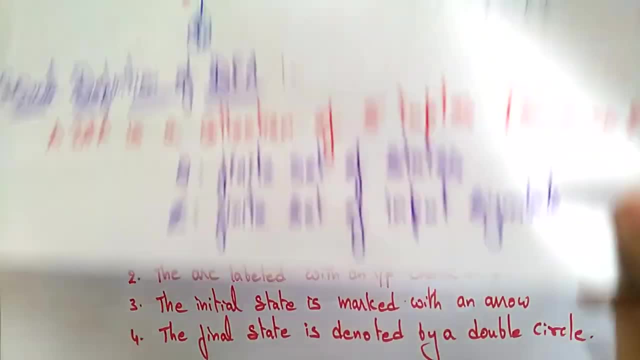 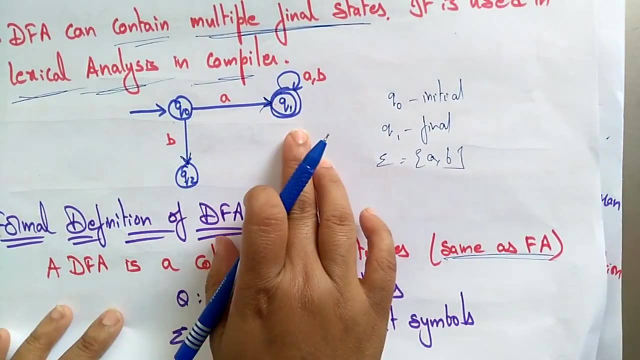 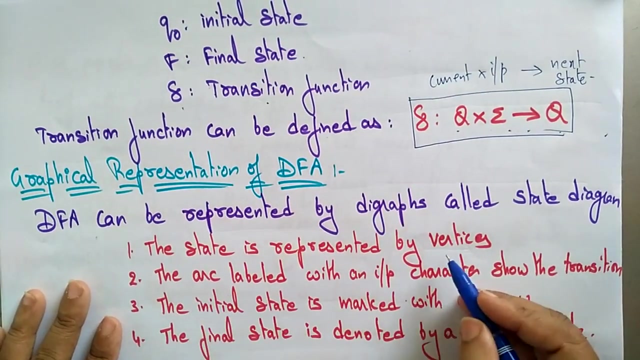 by diagrams called state diagram. so whatever you have seen, this is a state diagram. it's a digraph, means a directed graph. a direction should be there. from where, from which states? to which state? what state it is going on, on what input. so the state is represented by a vortices. 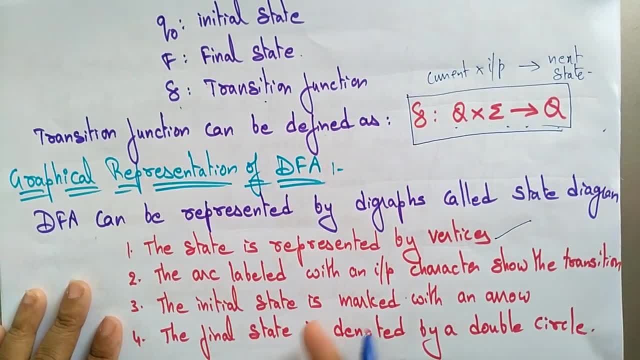 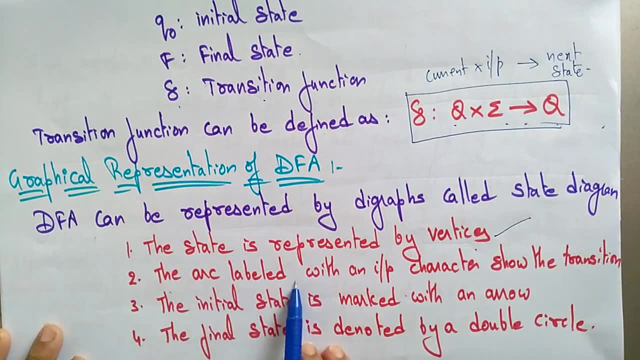 so here each state is represented by a vortices. let's put q0, q1, q3, lower, a, b, c, d, anything a state is represented by a vortices. the arc labeled with an input character shown the transition. so here the arc which is labeled with an. 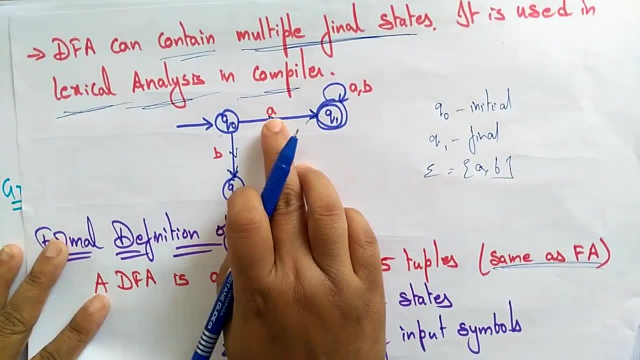 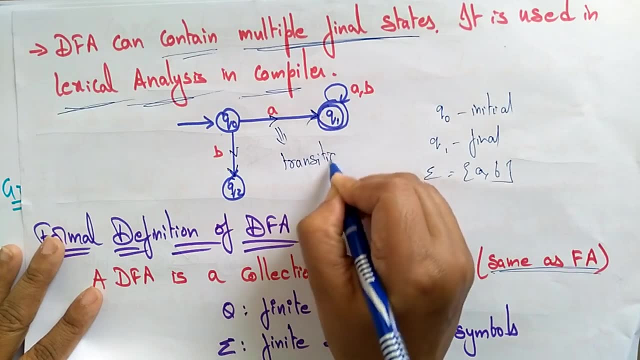 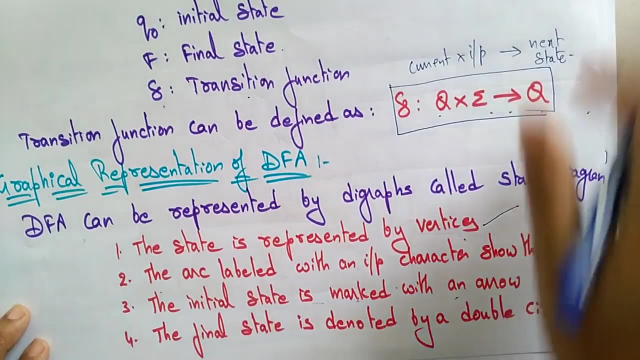 input character. this is an arc, okay, labeled with an input character, which is showing you call it as a transition. that's a transition. the arc labeled with an input character shows the transition. the initial state is marked with an arrow and the final state is denoted by the. 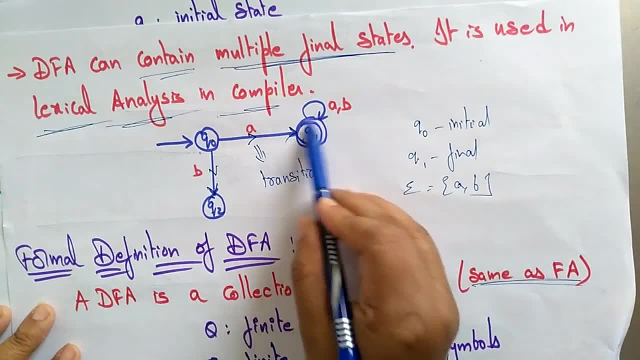 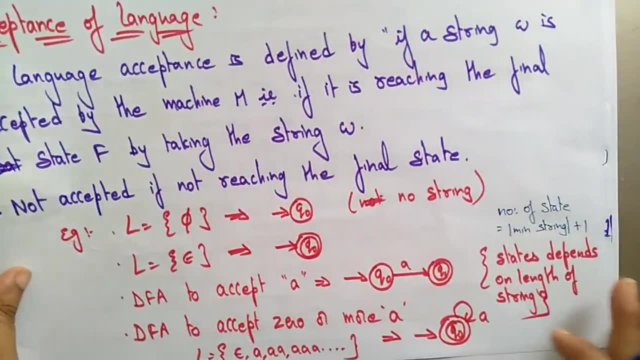 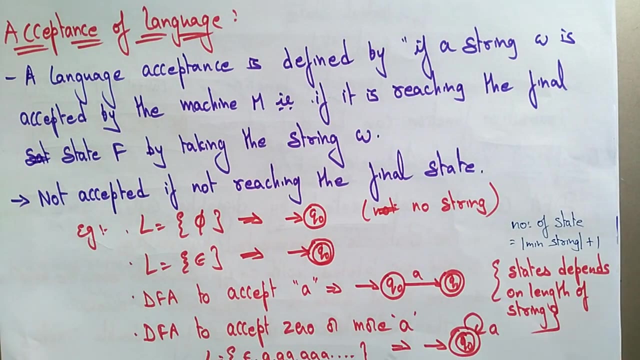 double circle. initial state is marked with an arrow and the final state will be with double circle. so this is a graphical representation of the digraphs. okay, so, uh, before going to the examples of this dfa, let me tell you what is an acceptance of a language. when you say the language, 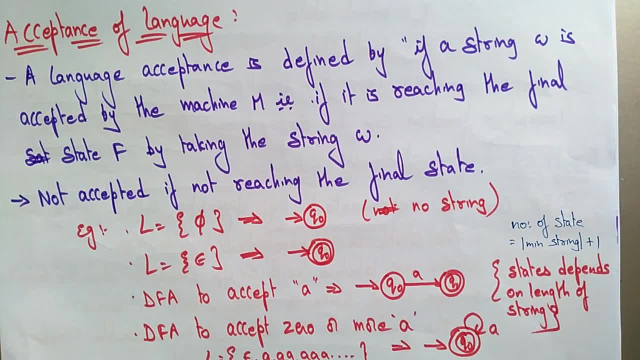 whatever the language that we are taking, that is accepted or rejected. i want to construct dfa. i don't know whether, whatever the string that i have taken, is it accepted or rejected. that i have to know. so if you want to know that, first see. what is this acceptance of a language? 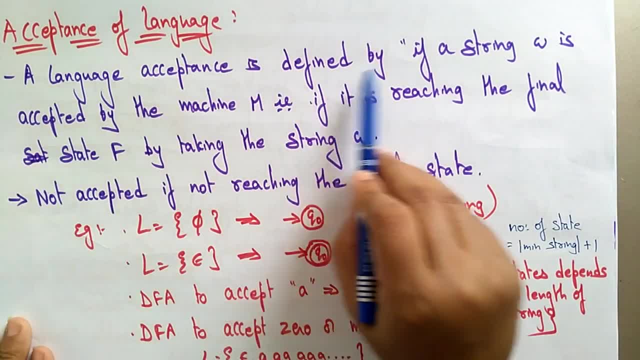 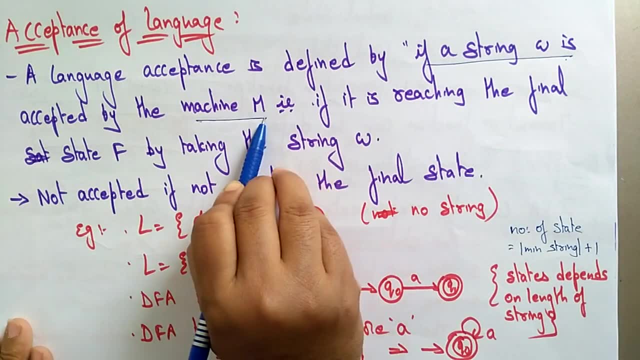 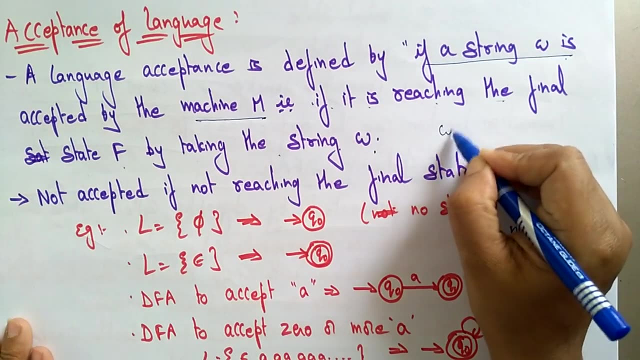 a language, acceptance is defined by: if a string w, whatever the string that we are taken, if a string w is accepted by a machine, m, that is, it is reaching the final state f by taking the string w. so whenever i have taken one string, whether something a, b, a, c, like this, so whenever, if it. 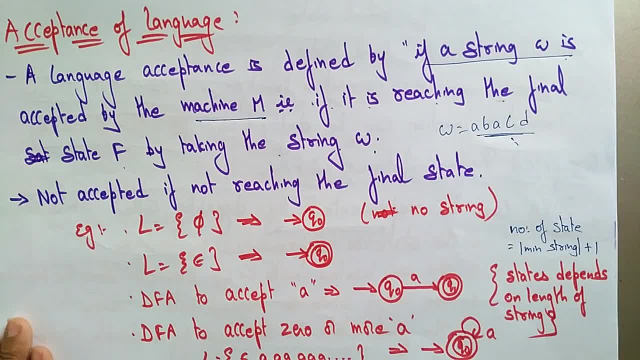 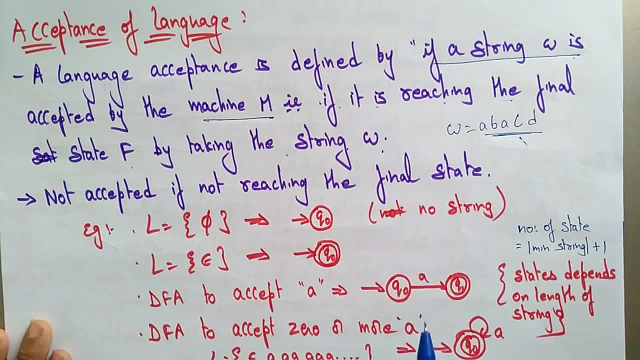 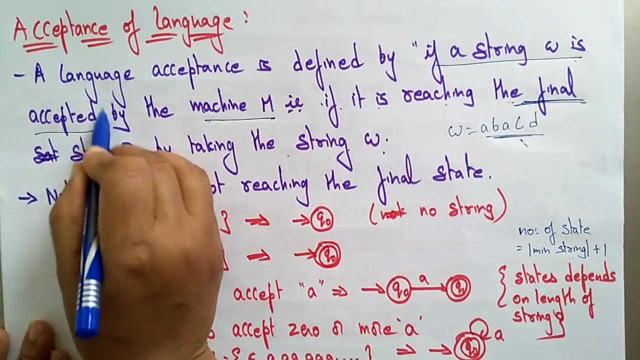 reaches the final state, then the string is accepted. otherwise the string is rejected. okay, not accepted means, if not accepted, reaching the final state. you have to remember that whenever the state reaches the final state, whenever the string reaches the final state, then you can say it is accepted, otherwise not accepted. 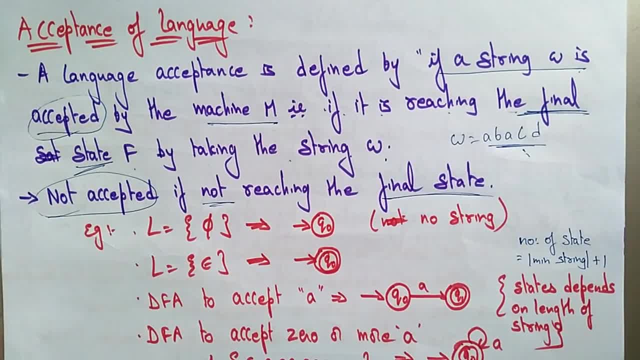 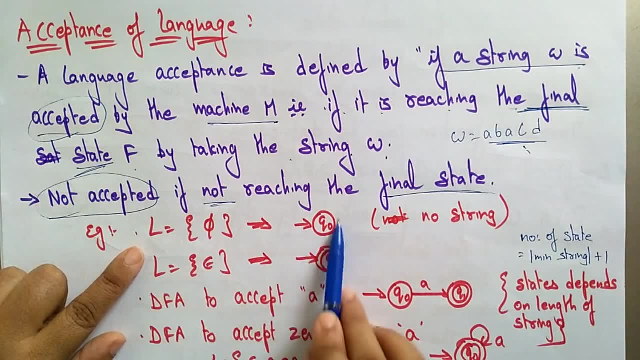 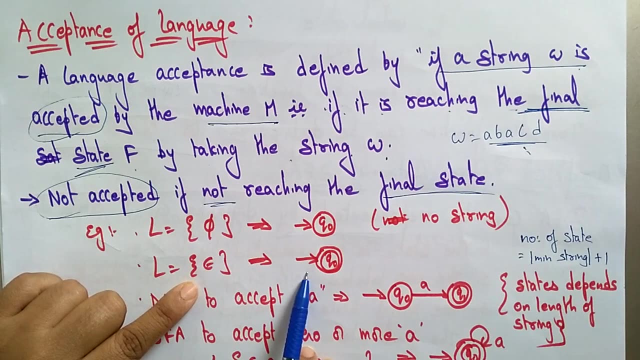 means not reaching the final state. so let me take the example. suppose if the language with phi means there is no string, is there only one state, is there q naught? there is no next state. and if the language with an epsilon empty state, it is a initial state and it is the final state. 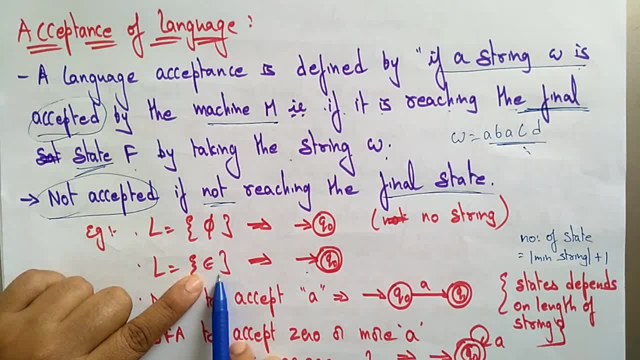 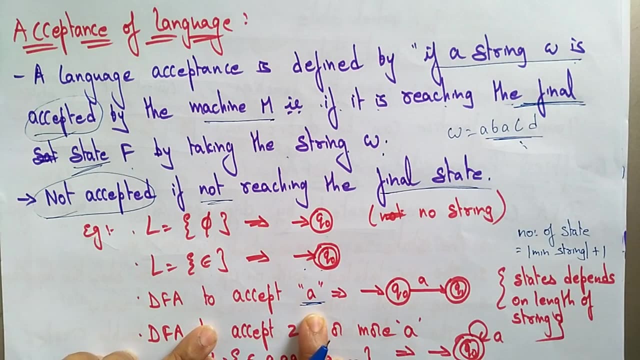 because there is no moves here, there is no moves epsilon. there is no moves means no transition, means it is this initial state as well as it is a final state. suppose dfa to accept a. i want to construct a deterministic finite automator which accept a, which accept a means. 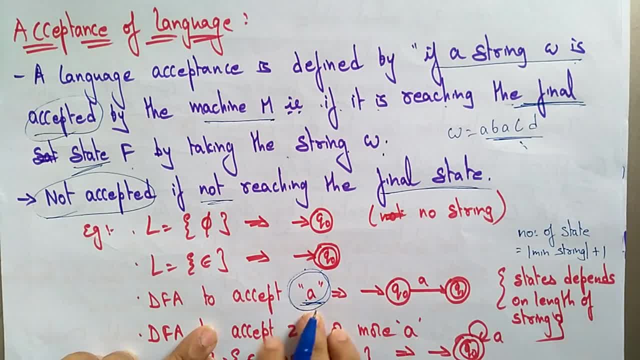 whenever first you have you need to check what is the length of the string that i have. taken you here the uh states, how many states i need to be. take you will get it out how i am going to construct the dfa diagram. okay, first thing, whatever the input they are given, the minimum. 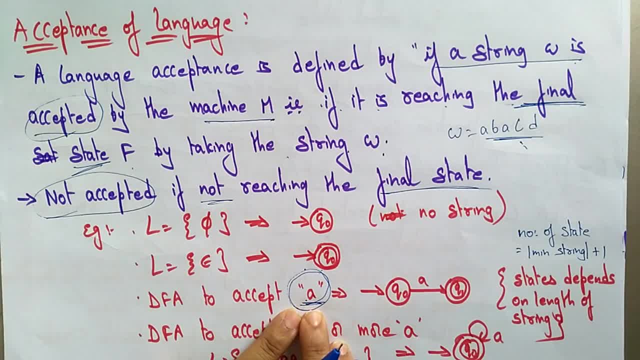 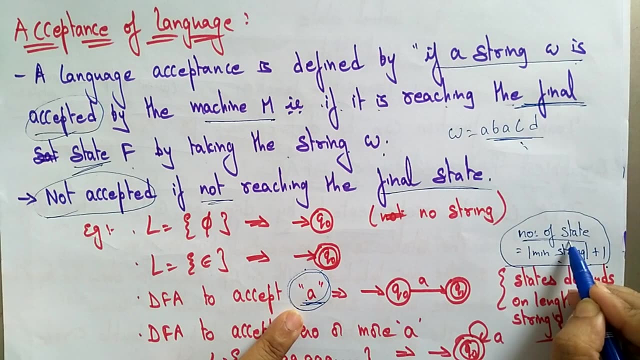 string you have to taken, it has to accept a means. this is the condition here. the minimum length of the minimum uh string length is one. okay, so the number of states will be. dip is depends on the minimum length of minimum string plus one represents the number of states. so here the straight. minimum string length is one one plus one two. that means two states are required. q naught q1. so the q naught on a goes to q1, which is the final state. so here this is the dfa which accepts the string a. the states depends on the length of the string. suppose if dfa to accept 0 or more a either. 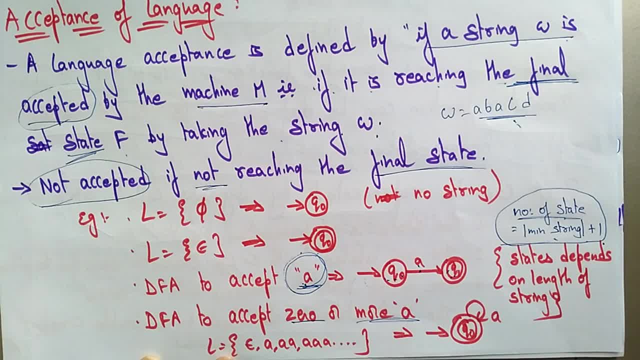 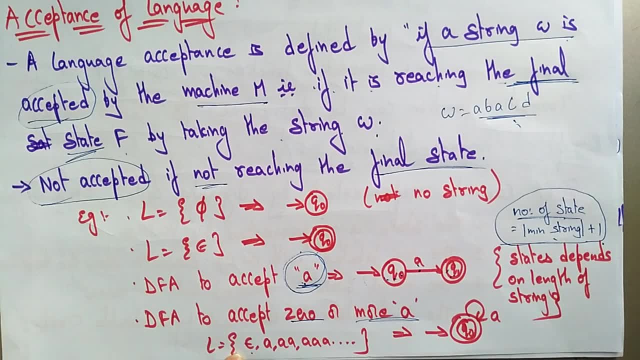 it has to accept 0 or it has to accept more number of a's. more number of 0 means epsilon. epsilon most means the string itself. you call it as an epsilon. a move that is taking place itself is except epsilon. more a, a, a, a, so like, so on, like this. so the dfa for this is: this is the initial state, with 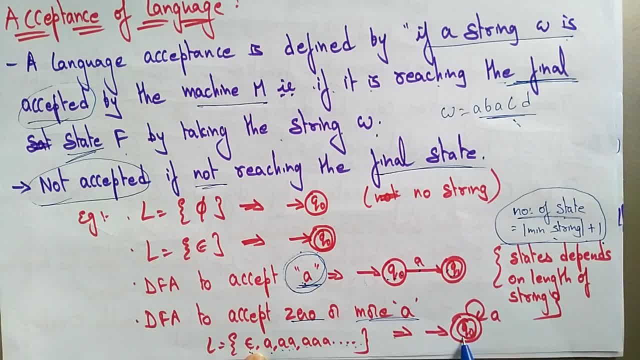 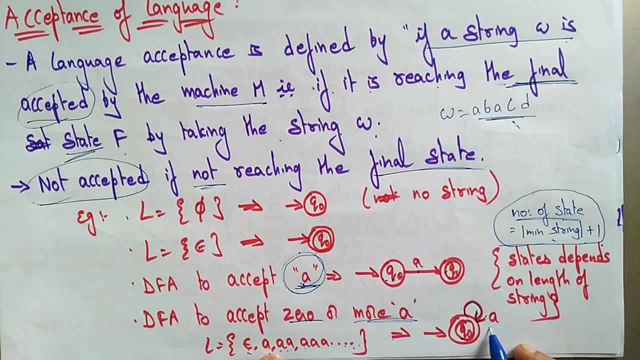 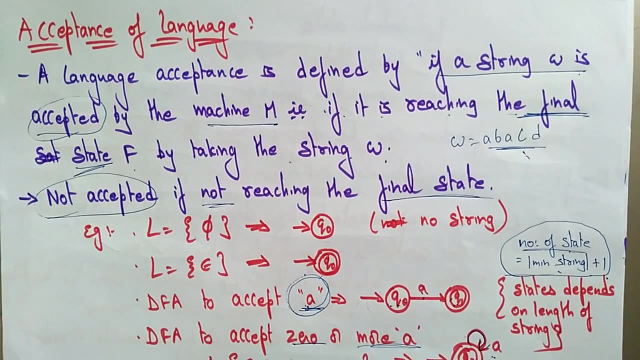 the accept 0. and this is a final state which is having a loop. so it gives epsilon moves a, a, a, a like this. so this is about the accept, acceptance of language. now i hope you understand what exactly the dfa. so in the next videos i'll